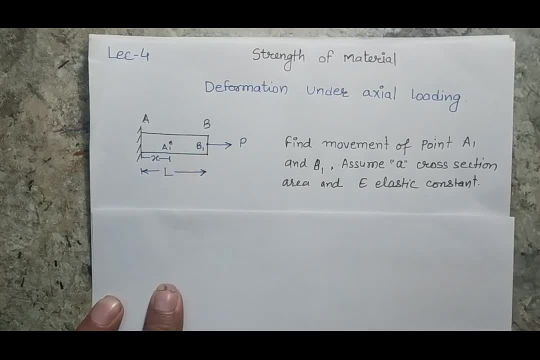 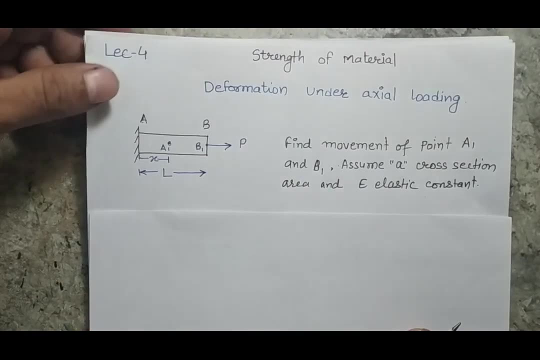 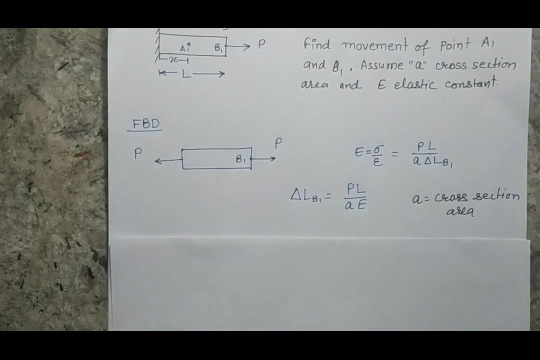 deflection of point b1 as well as point a1 will be same or not. so surely the deflection of these two points will not be same. the deflection of these two points will be different, but how these two deflections will be different. let's see that suppose. first thing which i need to do is to find. 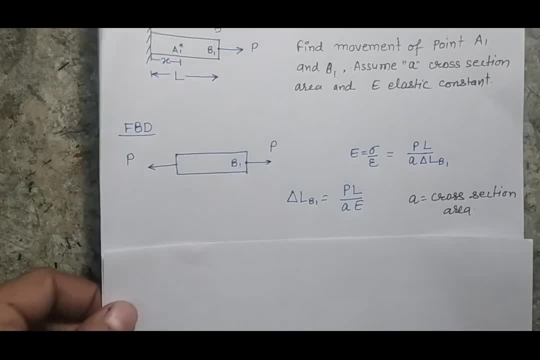 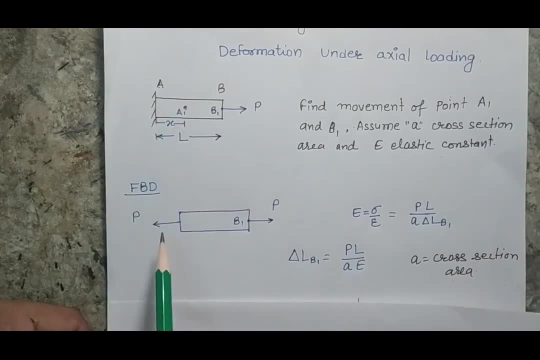 the free body diagram of the complete bar. as i know that there is only one force acting at this point, then the support has to apply equal and opposite force to this end, so that i have made a point p here which is acting opposite to the point p and equal to the. 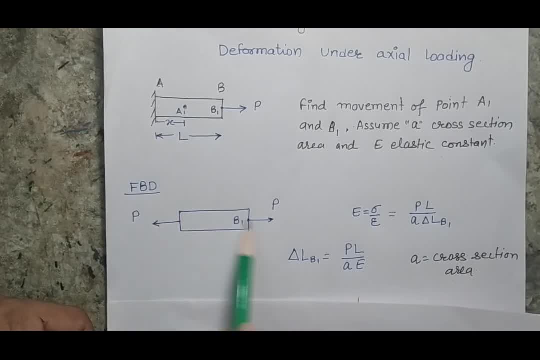 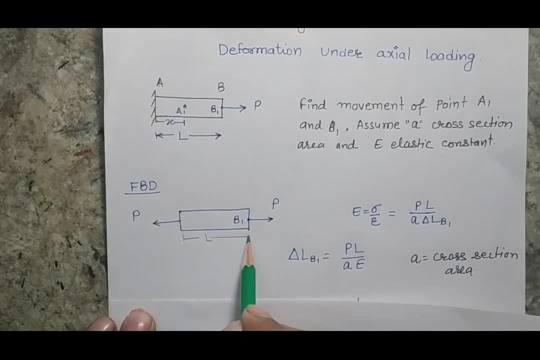 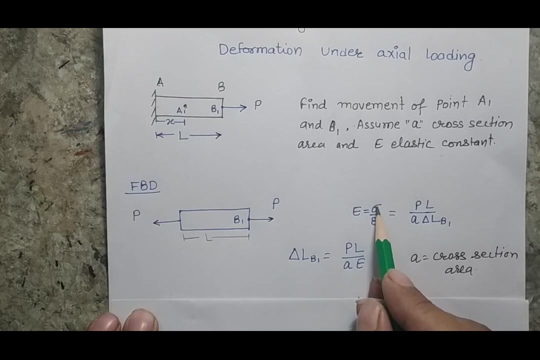 magnitude of force opposite to this force and equal, also also equal in the magnitude. so now, as i know that this is a body of length l and i am applying a force p on the body, so so i know the relation, that this is the elastic constant, which is the ratio of stress by strain, and i am 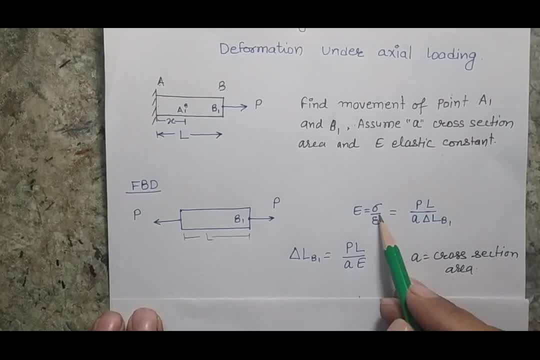 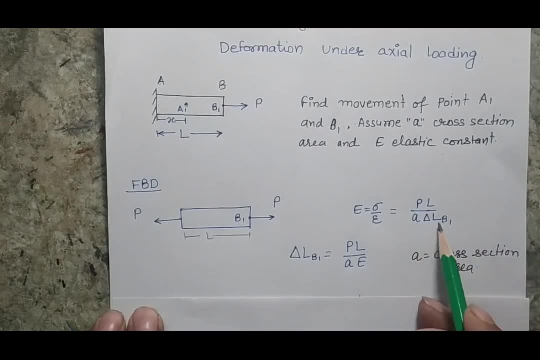 talking about the one dimensional stress and strain. so my stress will nothing but the force by the cross section area. here a is your cross section area, and strain will be change in length divided by the total length. so i have moved the total length on the numerator side. so now this: 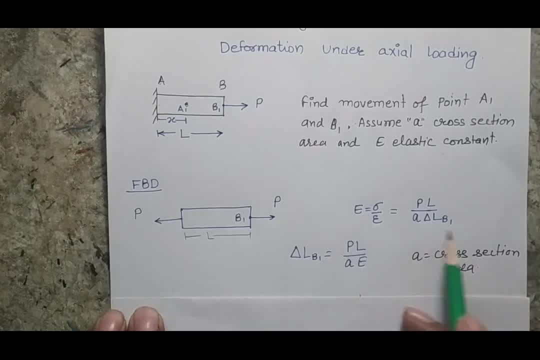 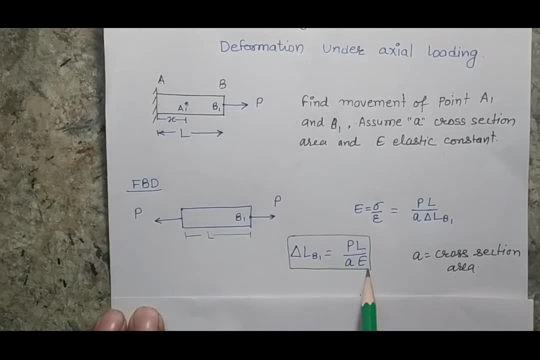 is my formula for the elastic constant and if i will rearrange the term i will get this formula, which is very basic formula and we are going to use this very frequently. so if i am interested to find the change in length of this bar, my formula will be basically the force applied. 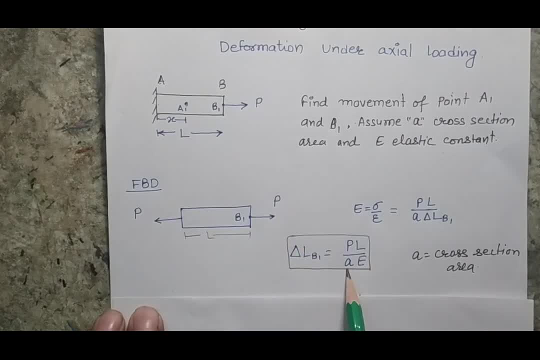 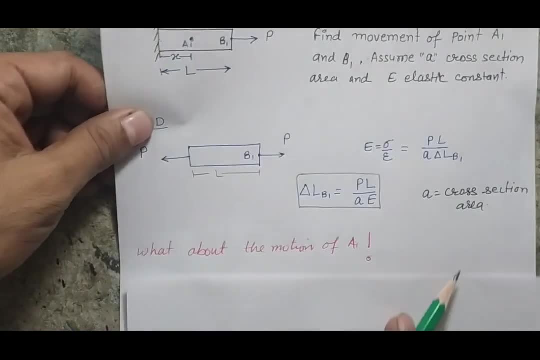 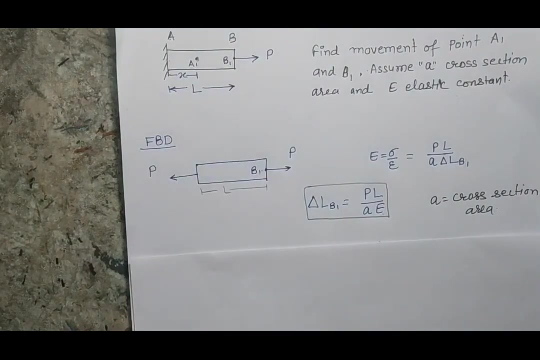 to the bar, then the total length of the bar divided with the cross section area and the elastic constant. when i apply this formula to this bar, i will get the deflection of my point b1 with respect to the fixed point. but now, what is the deflection of point a1? so for that i first. i am going to first. 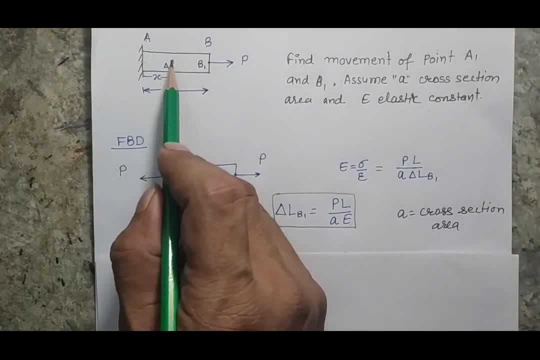 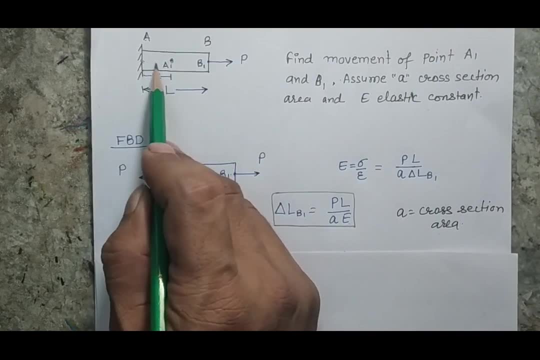 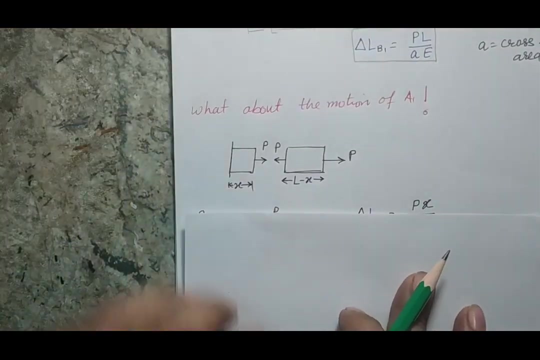 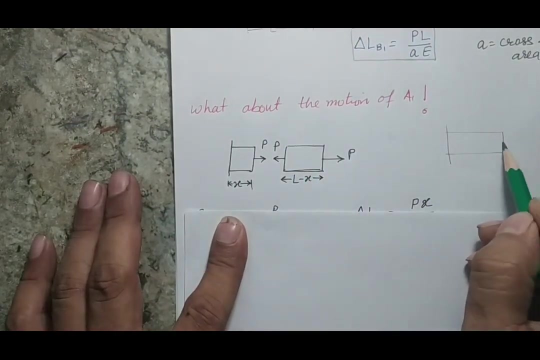 find that what would be the force acting for this section? because whatever force will be acting, this section is responsible for the change in length of the section. so if i will break my bar at this point and make the two free body diagram, i will find that now i have broken my bar and i know that if i will see that this is my bar, i am applying. 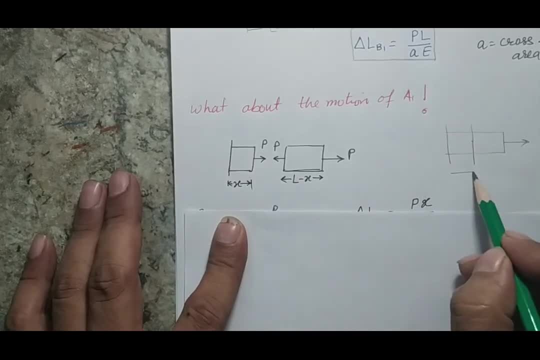 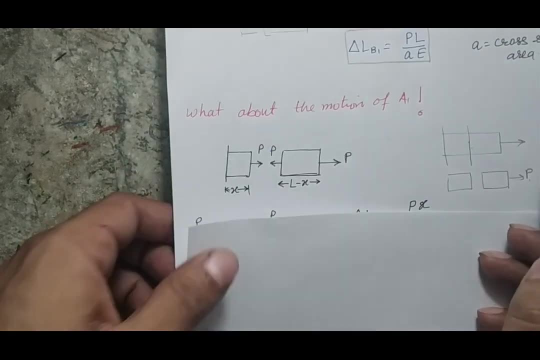 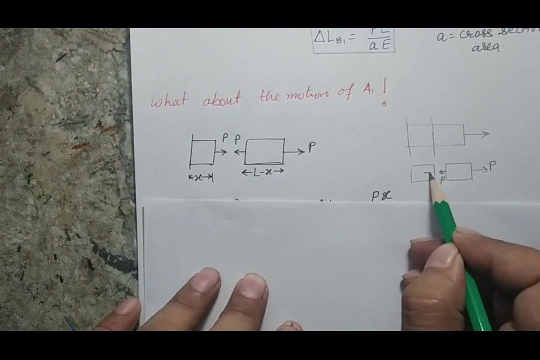 certain force here and suppose i am breaking my bar at this point. so, as this, this section, should be in the equilibrium, i know that force, whatever force acting at this point will be balanced by the force acting on other point and as this is the force b, the equal and opposite force will be applied by this. so ultimately i will get that the 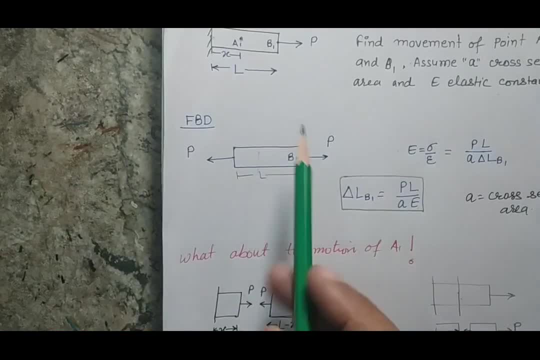 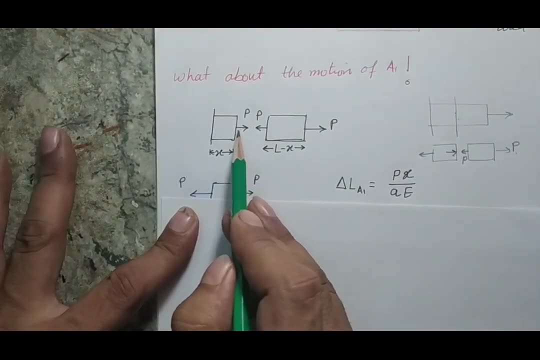 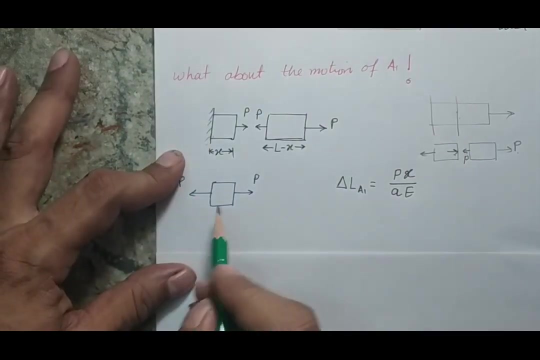 force will not going to change throughout the bar and the complete bar is experiencing the same force. so now, now i am having the small section and i know that this portion is having a force p, so equal and opposite force will be applied by this fixed support. so now, this is the diagram for 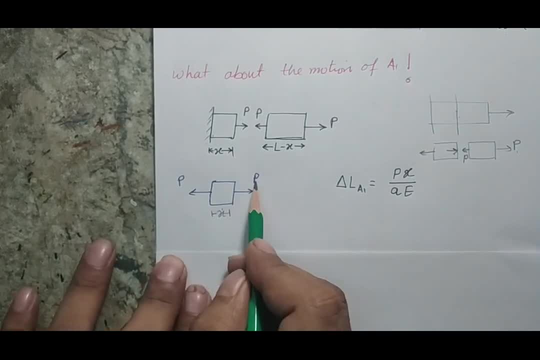 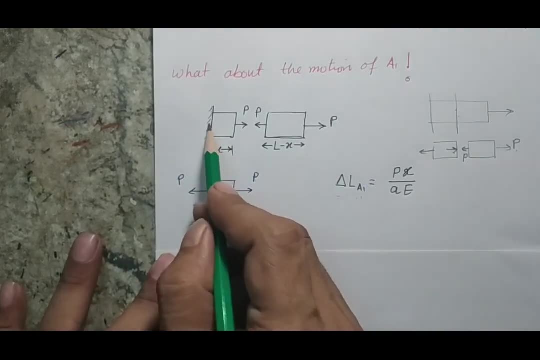 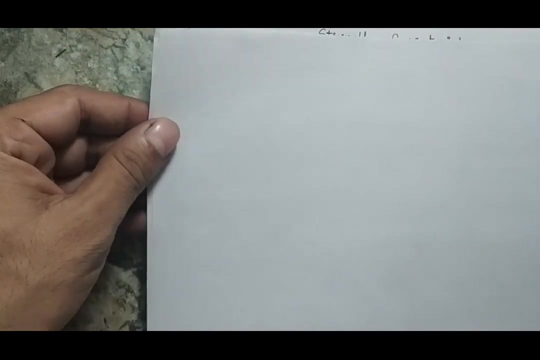 this small x length bar and if i will apply the force p for a length x, i will get the change in length or the motion of the point A with respect to the fixed end will defined by the term PX, by AE. Now let's take another problem which give you an insight: that if 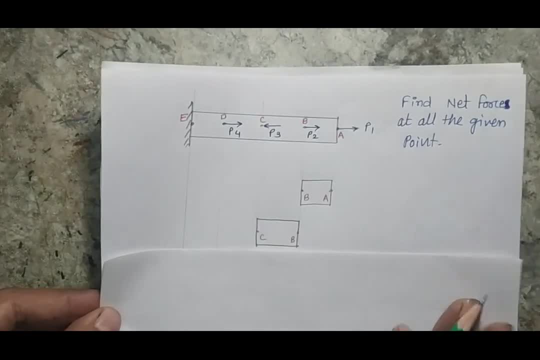 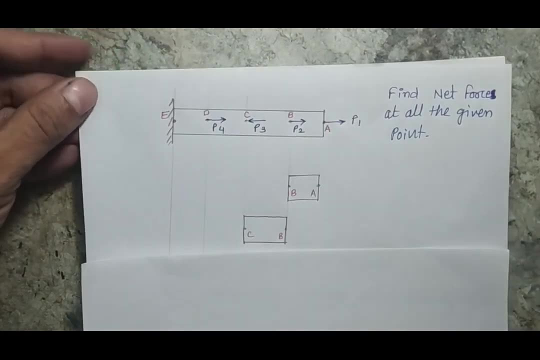 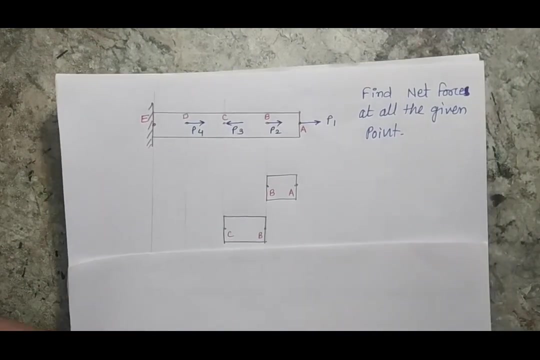 you are having number of forces on a bar and you are interested to find the forces in each section of your member. Here I am going to tell you one simple trick so that you won't have any problem to calculate the forces in the individual member. For example. I am showing: 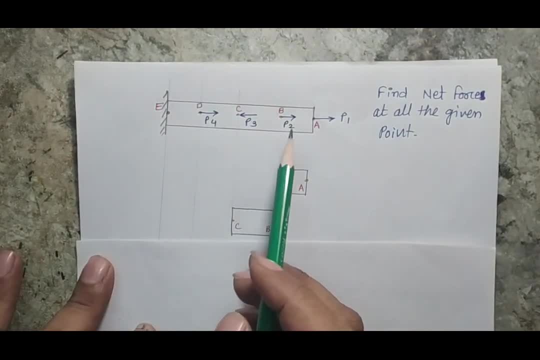 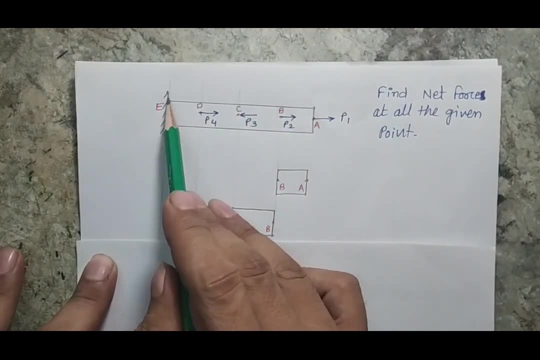 here a problem where I am having a long bar and I am applying four forces: P1, P2, P3 and P4.. I have shown point A, B, C, D and E. The end E is the fixed end and end A is a free. 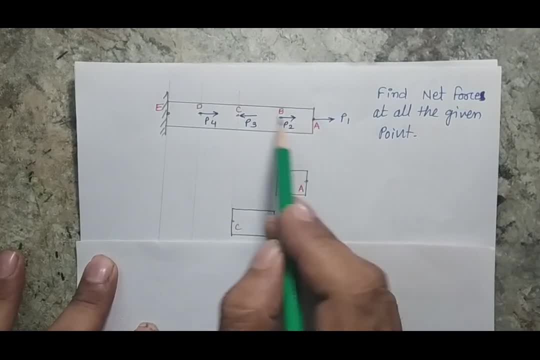 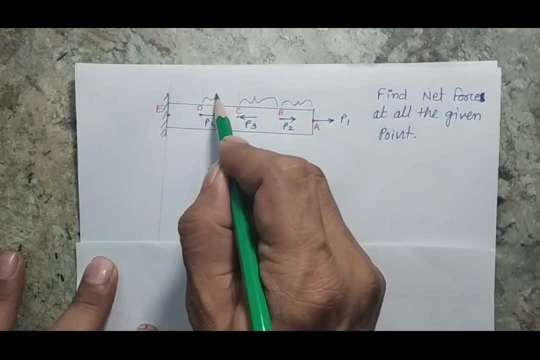 end, and I am interested to find the forces in each section. So suppose this is my one section of the bar. This is my second section of the bar, as well as third, and so on the fourth one. so first what I did. I have drawn the. 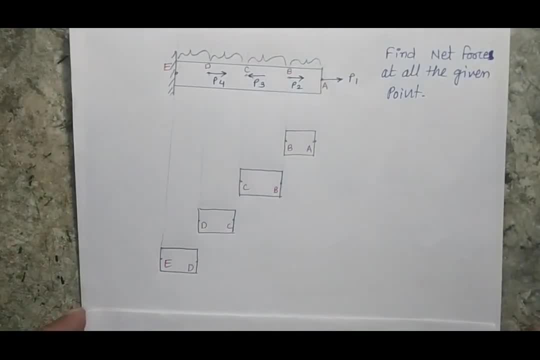 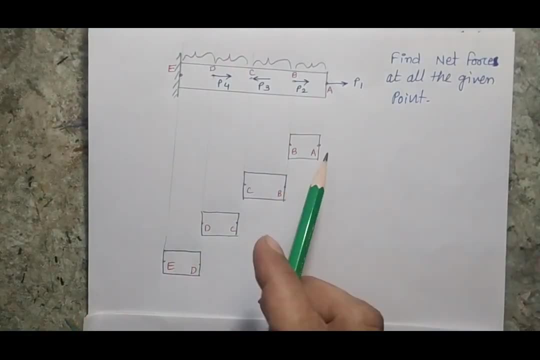 fourth section here. you can see here now this is the complete picture in front of you. so here what I can. I can start the problem either from this side or this side. as I know the force at this end, what I will do, I will apply this force. P. 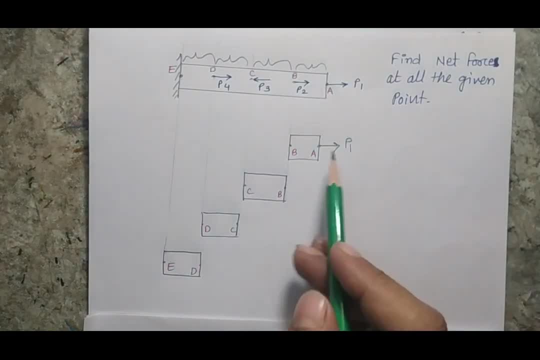 as it is here, P1. I am NOT bothered that what will be the force at point B. I will first make the force P1 because this is the known force to me which is acting at point A. now, if I will see this portion of the bar, I can say: 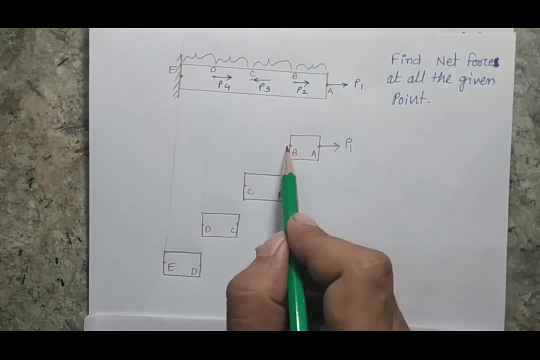 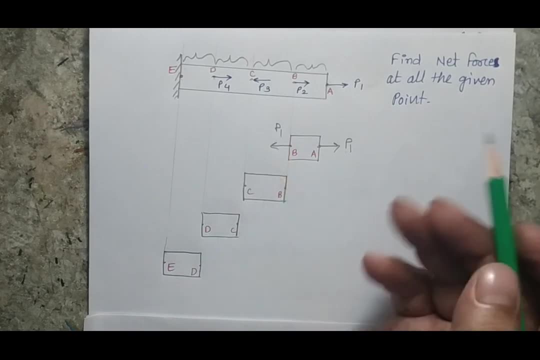 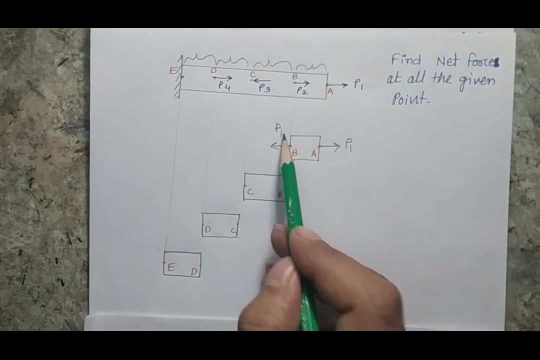 that this should be in the static equilibrium. that means whatever force will act on the opposite side should balance this force. so it will be P1. you made the, you make the force P 1. irrespective whatever forces are given at, different forces are given here now. now this P1 force is basically: 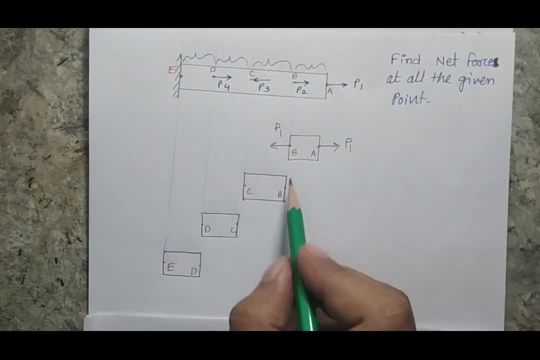 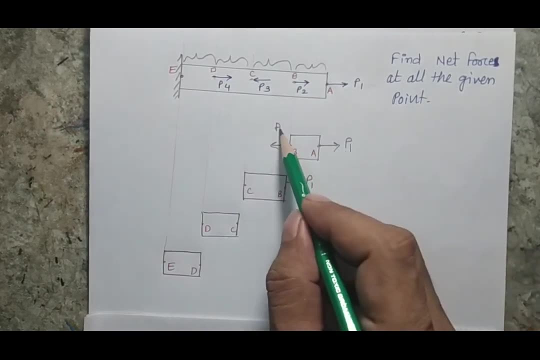 generated by the made force P1. this forces generated by doing this exercise because of the remaining portion of the bar. that means I am going to apply a P1 force here also. and now what I am saying? I am saying that this P1 is applied by this portion on. 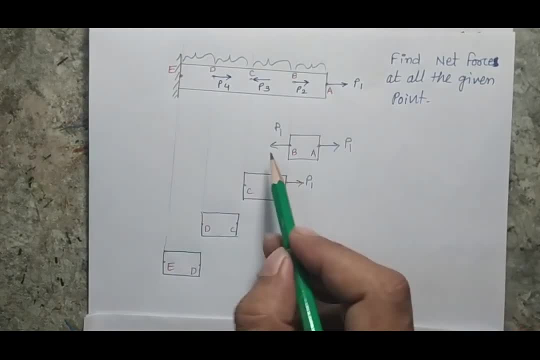 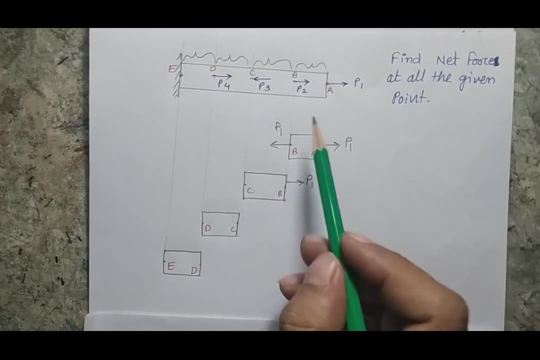 this part. so similar, equal and opposite force will be there. so this P1 generated by this section. so this P1 is generated by this section. this is Newton's third law. so this is P1. now I will see that. is there any more for other force here? so yes, there is a force of P2. so 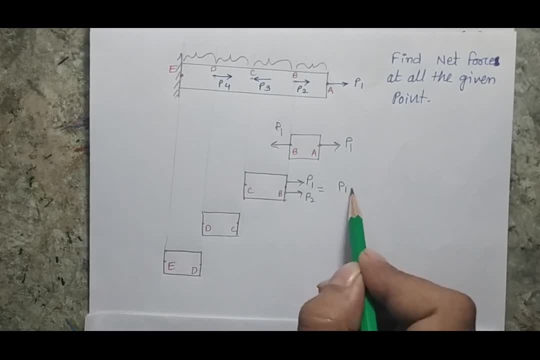 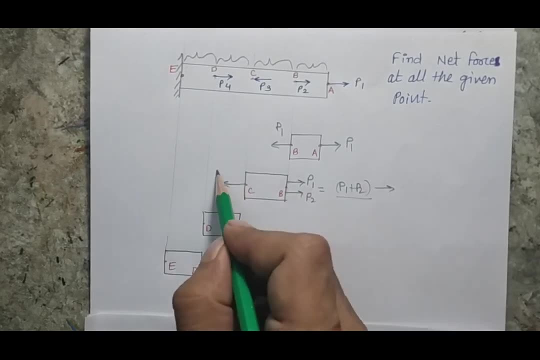 ultimately, the resultant of this T is a force which is having P1 plus P2 value and that acting in this direction. as I know the force on this side, simply I will put equal and opposite force here. so I know that this is P1 plus P2. now, as this is P1 plus P2, I know that this. 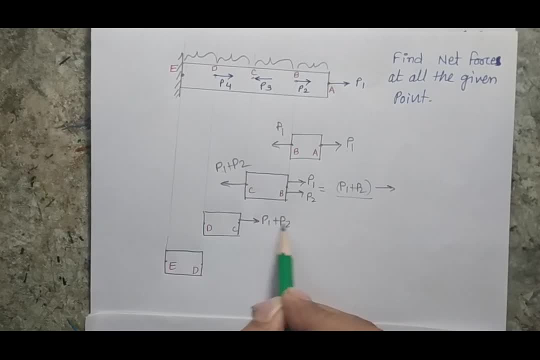 P1, P2 is generated by this section, so I will put one P1 plus P2, and now I will see any other force is one force- P3- here, so I will put another force, P3- here. so net force on this side would become P1 plus P2, minus P3. 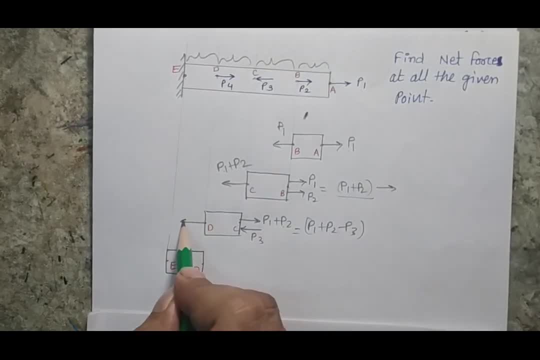 Similarly, this is minus P3. I will put equal and opposite force here, so it will become P1 plus P2 minus P3. now the same will act here, so it will be P1 plus P2 minus P3, as well as one more force. 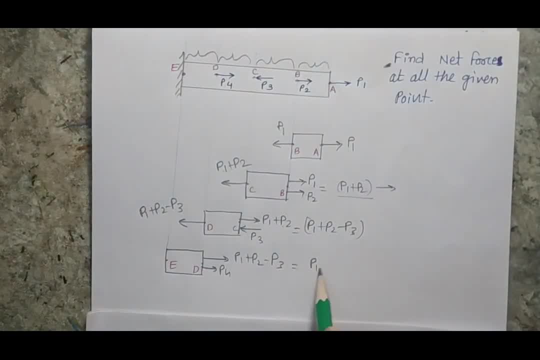 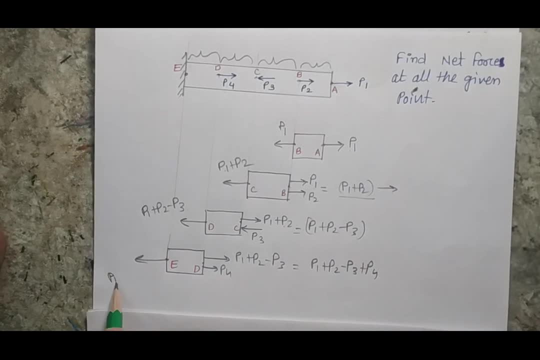 is acting here, so I will put P4. so my net force will be P1 plus P2 minus P3 plus P4. so the same force will act here. so this would be P1 plus P2 minus P3 plus P4. so in this: 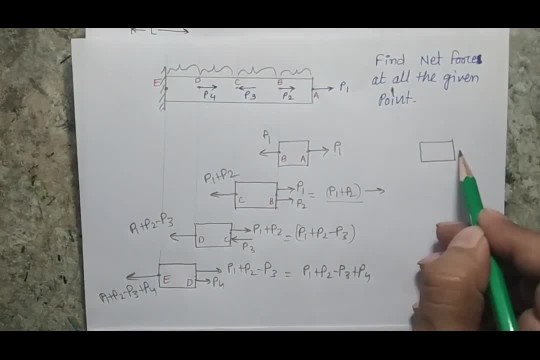 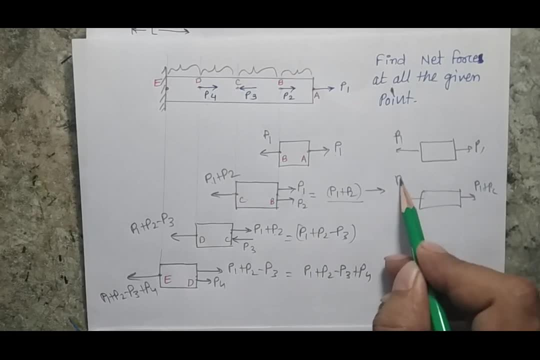 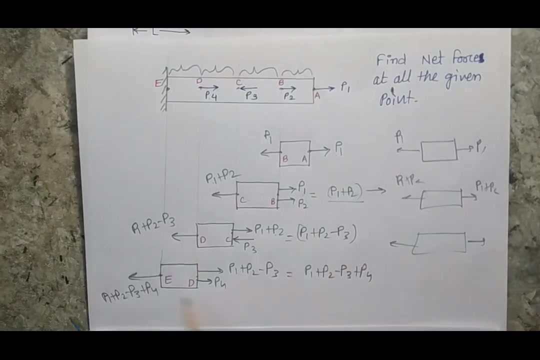 case I am able to get that, the net force on the first section will be P1. for the second section it will be P1 plus P2, similarly here also P1 plus P2. for the third section it would become P1 plus P2 plus P3 and P1 plus P2 plus P3, and for the fourth section it is also P1. 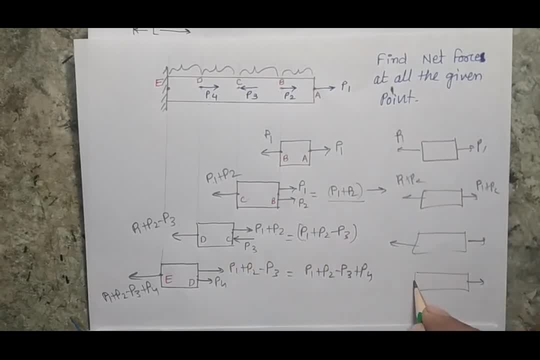 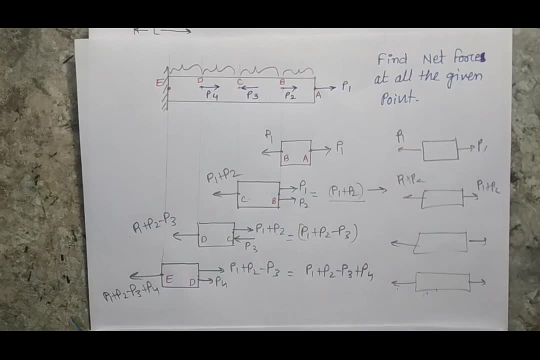 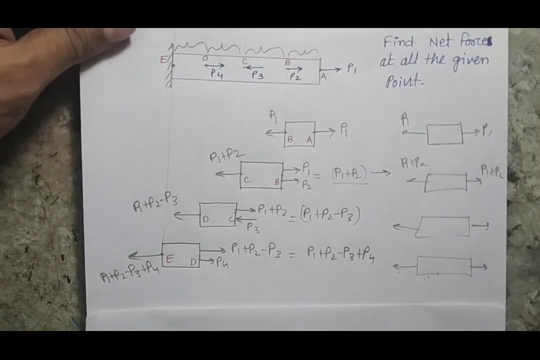 plus P2 minus P3. sorry, here it will be also P1 plus P2, minus P3 plus P4 and the same value. So now, based on these Analysis, I can calculate the forces in the individual member. and once I know the force in the individual member, I, if I am interested to find the change in length, I can also calculate. 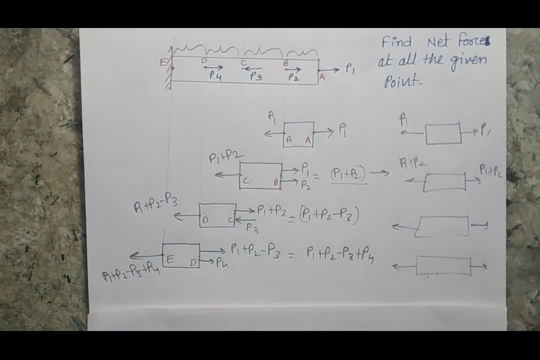 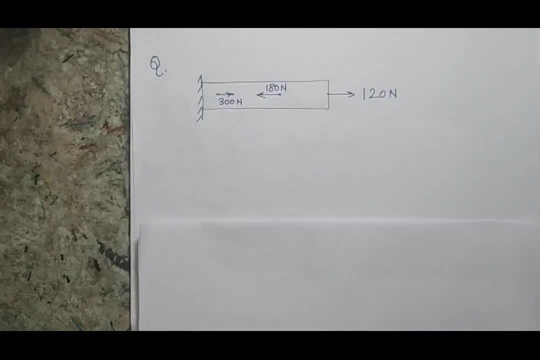 the change in length in individual section. that problem we will see later on. so to repeat the same, I'm just showing one numerical problem here. I am showing that there are three forces acting on this member. so let's put that: this is point A. now this is Point B, this is point. 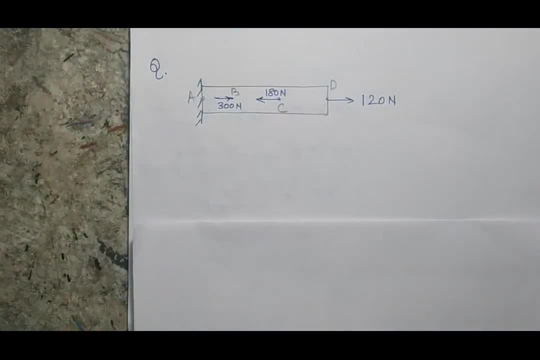 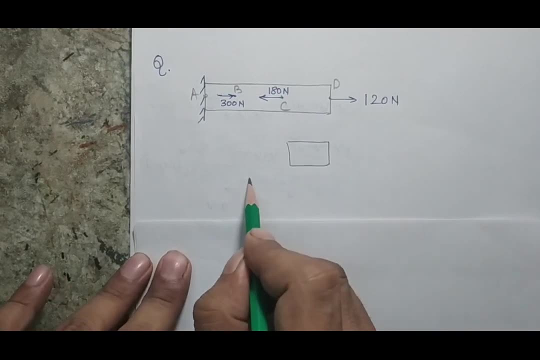 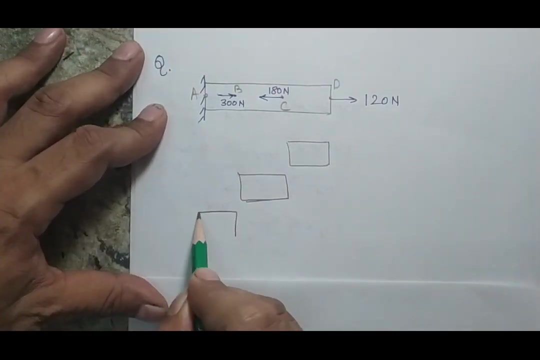 C, and this is point B, and I'm interested to find the forces 2. forces in each section. so what i will do? first i will make this cd part, then i am going to make this second, which is your bc part, and the last i am making the section which is your. 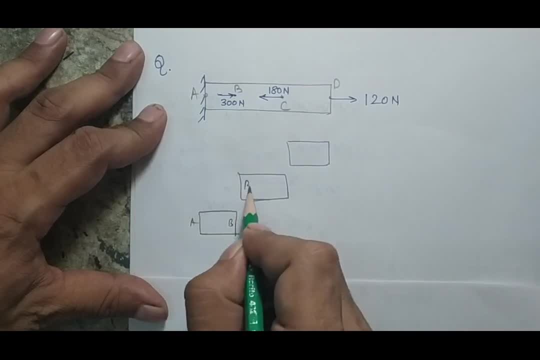 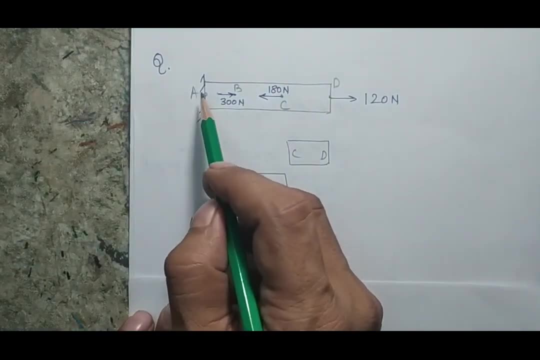 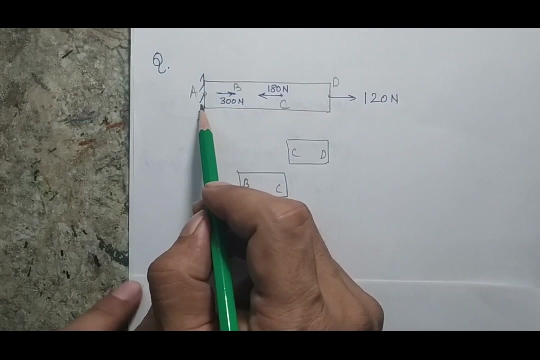 ba part. so this is ab, your bc and cd. as i know, this is 120. you can start from this side. otherwise, if you want to start from this side, first you have to find the force at this end and the forces at this end will be equal and opposite the remaining forces acting on the bar. so if i am interested to 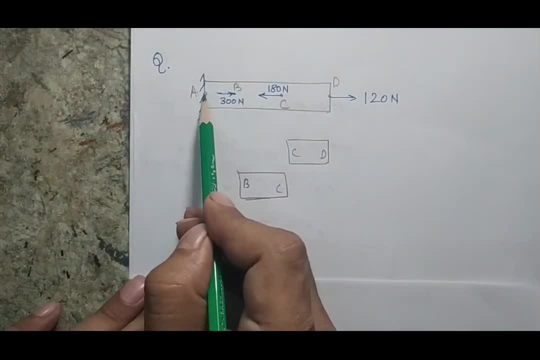 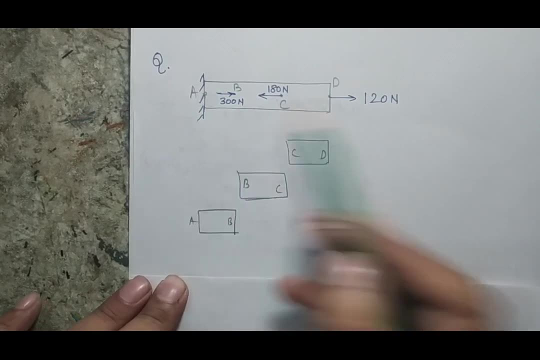 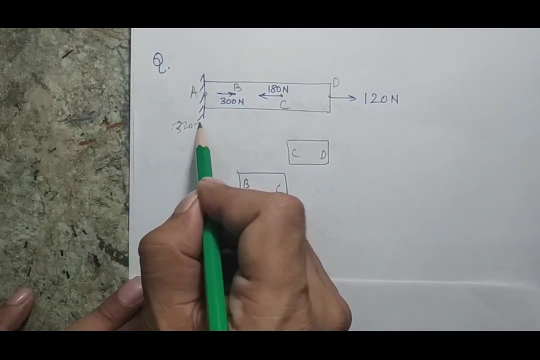 find the force in the beginning. i can check that the total force at this section is going to be balanced, all the other forces here. so it is 120 rightward, 300 rightward, so 420 rightward but 180 towards the left side. so ultimately the force will be. here will be the difference of the 320 minus. 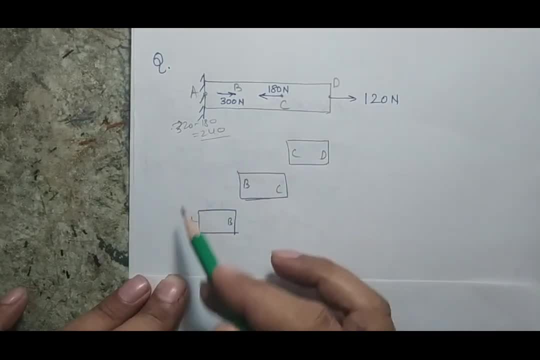 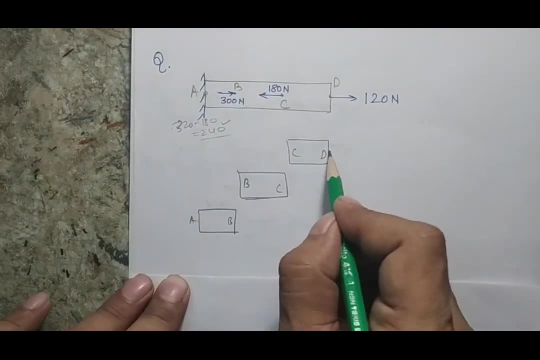 180, that would be 240 later on. if we will solve the problem using this philosophy, we will. we will be able to get you that, whether the answer is coming to 40 or not. so let's start that this is 120 here, as this is 120. 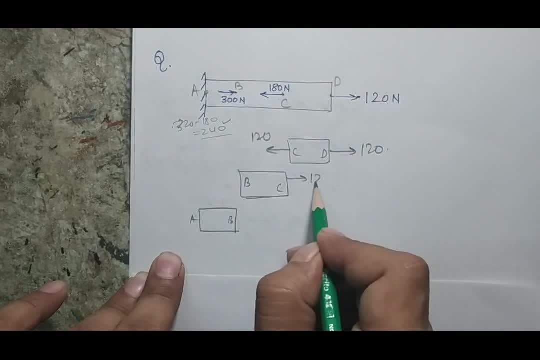 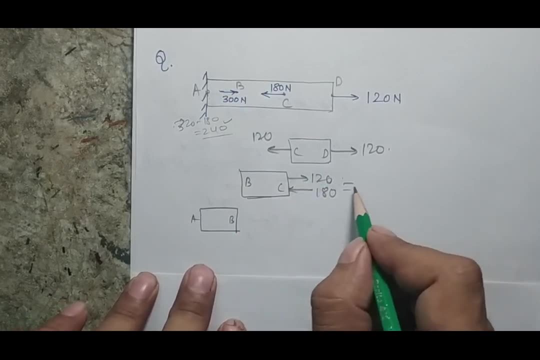 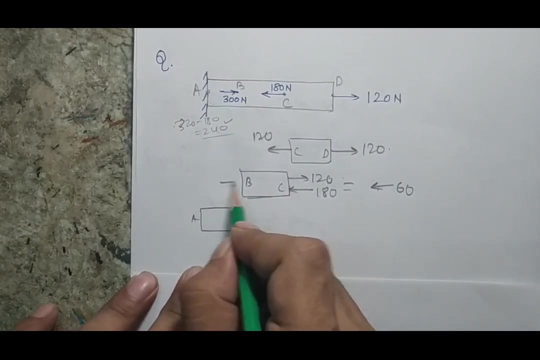 it would be 120. now this 120 because of this section, so it is 120 and additional 180 is acting here. so net force will be what? net force will be? 120, this direction and 180 is this direction, so net force will be 60 in this direction. so as 60 is a compressive force, i am putting a 60 here. 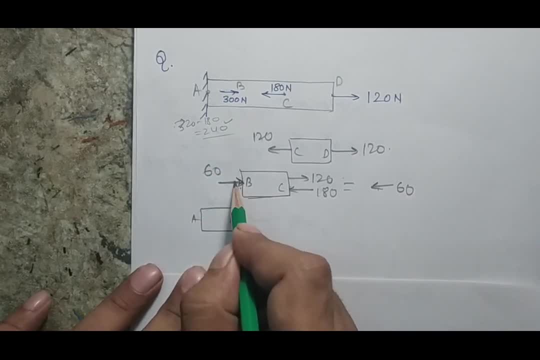 now this way. so this is six direction of the 60. now change to equal and opposite direction. i am going to put here: so this would be my 60 and the 300 is acting in this direction. so this is 300. so ultimately it would become the 240 in this direction, as 240 in this direction, equal and 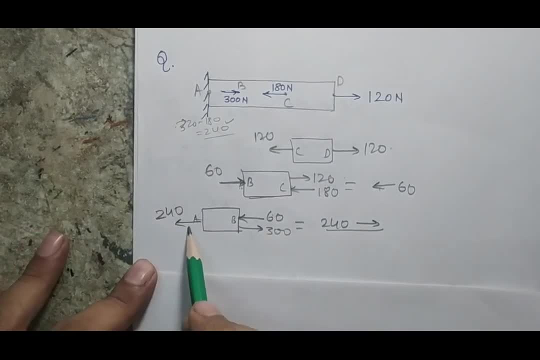 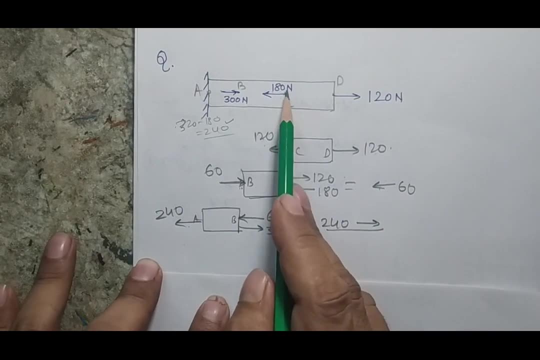 opposite force. so 240 will be here so i can check that this is 240 is matching. i am repeating here that what happened for the first section it was to 120, 120, but as i have observed that this section having another force of 180, so when i am doing an algebraic sum, i am getting that my answer will be: 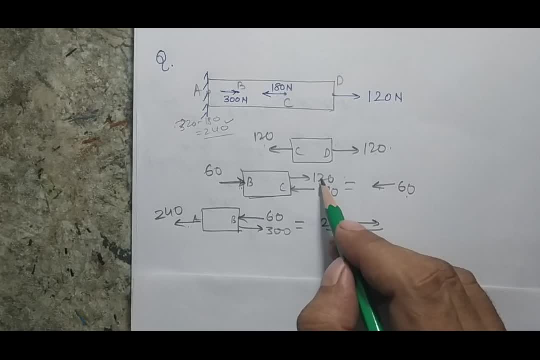 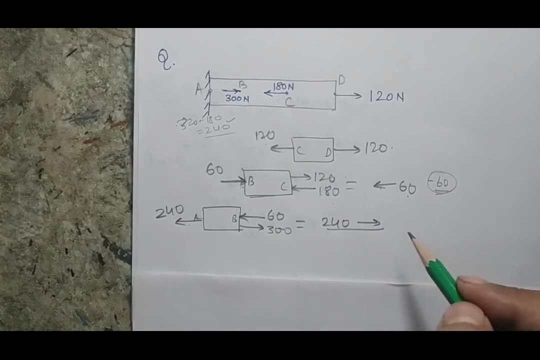 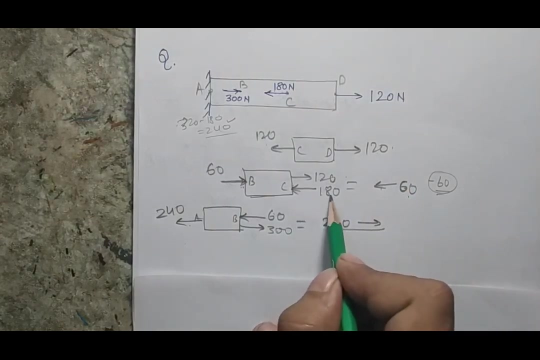 60 or minus 60. if i am taking 120 positive and 180 negative, my answer will be minus 60. that means it's a opposite, for this is basically the compressive force, or, instead of that, what i can do, i have simply made the direction by taking the actual direction, that is, 180 is towards the left. 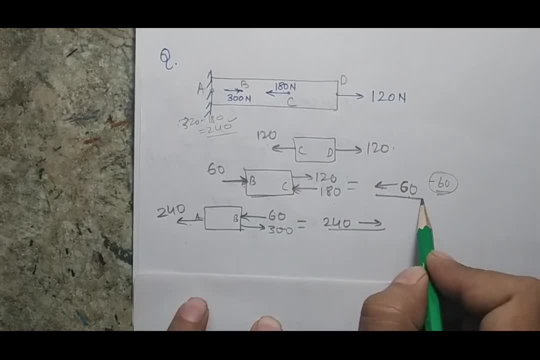 and 120 towards the right, so net will. so net will be one six only 60 inside the body, so equal and opposite: 60 here. this is 60, so i have to make equal and opposite here. so this is 60. 300 is already here, so i am getting a 240 net force. so in that way you can find the forces in different. 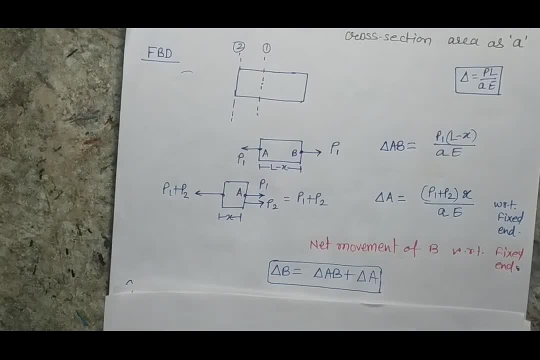 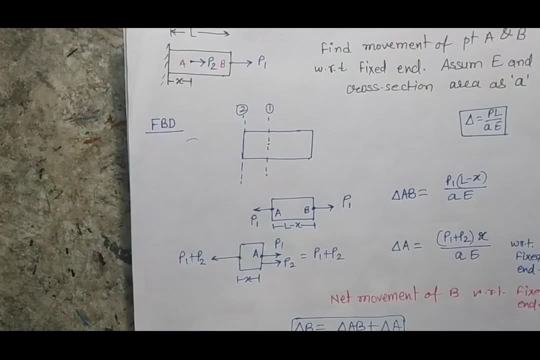 member so quickly solve a problem. this is, uh, another case where i am showing that, that there is a. now there are two forces which i have already seen in my previous case, and here i am interested to find the change in length. in addition to the finding the forces, i am also interested to find. 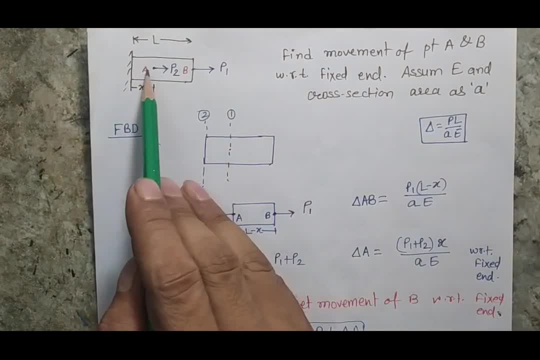 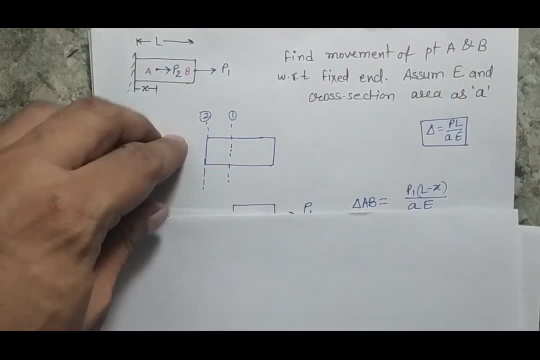 the change in length. so quickly see this problem. now we are having two forces, p1 and p2. the total length is x and there are two points. one is at distance x, another i am showing at the at the end. so this is my problem and i am interested to find. 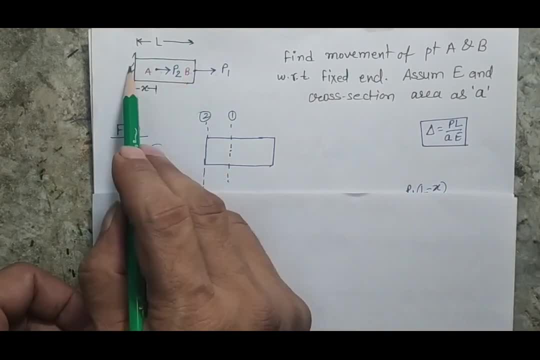 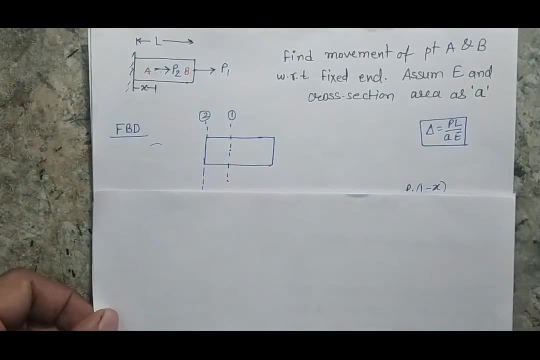 the movement of point b with respect to the fixed end and movement of point a with respect to the fixed end. so i know that if i am interested to find the movement of point b i first, i should first know that what is the forces in this part? so let's make the two parts. 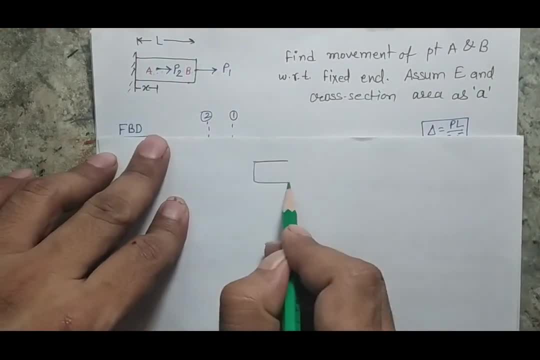 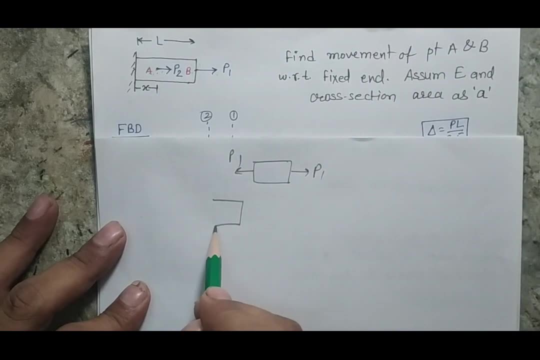 one part. i am going to make that. this is my one part. this is force p1, so this would also be p1. and when i am going to make the second section, this is the section for length l minus x. this is the section for length x. so now this is p1, p1 and for the other section it would be p1 as well as. 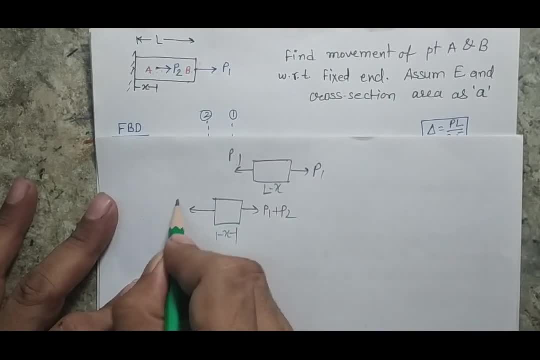 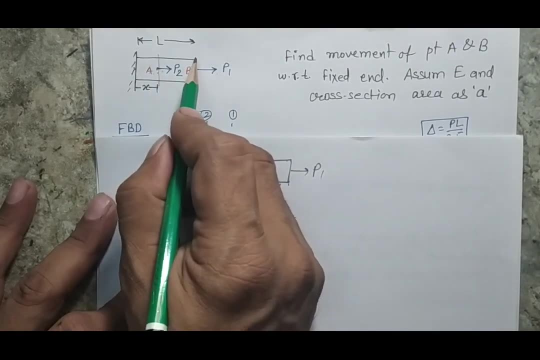 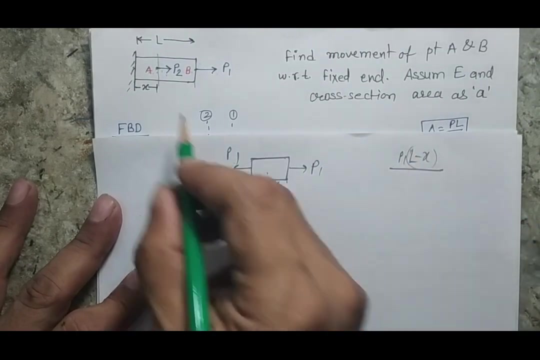 the p2. so i am directly writing p1 plus p2 and this would be p1 plus p2. now if i will calculate the change in length for this section- for this section i will get, my change in length will be what p1 and the total length, that is, l minus x, divided by 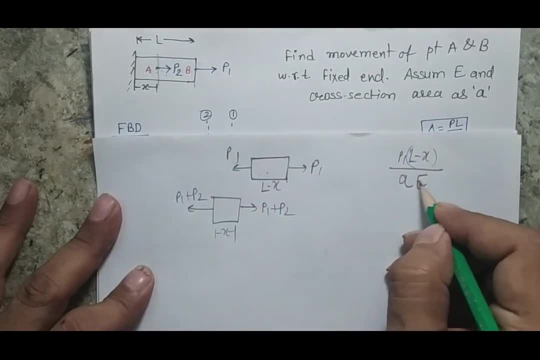 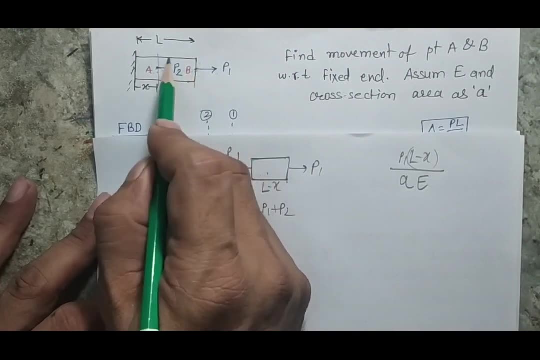 the cross section area of this body, a, and the elastic constant let's e. so this is the change in length of this portion and, as this is going to extend ultimately this that this portion will going to increase the length. now, for when i will check for the second section, i will get that the 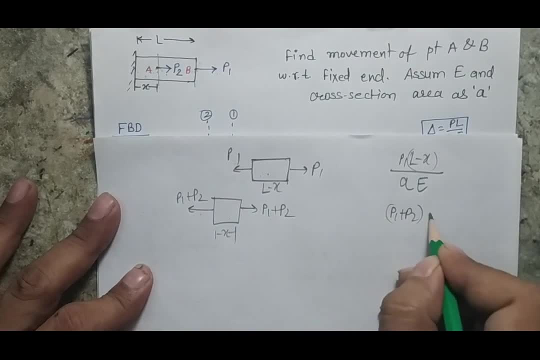 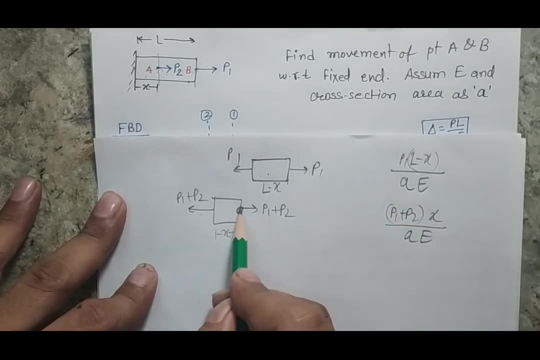 change in length for this section would be p1 plus p2, then the length x divided by the cross section area of this section. so this particular section, whatever change in length for this point, is basically giving the net deflection of point a, which is here. but if i am interested to find the 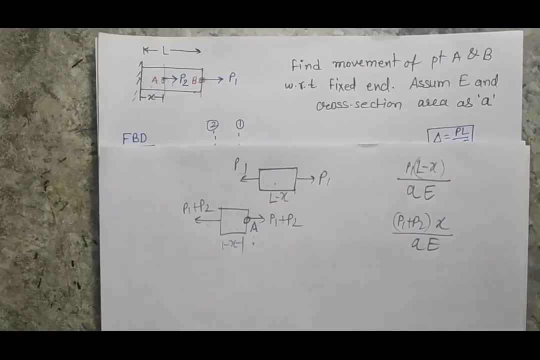 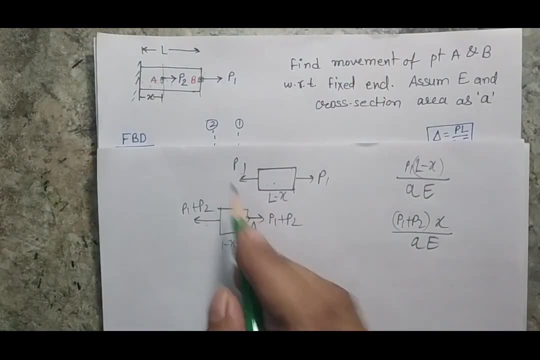 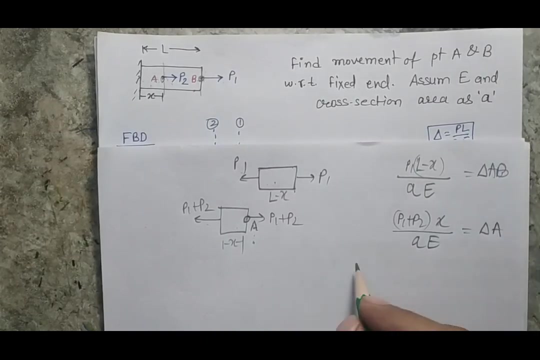 deflection of point b, the deflection of point, summation of the deflection of point a as well as change in length of a b. so, ultimately, the deflection of: if suppose this is the change in length of a b and this is the change in length of a. so my, ultimately, my final answer will be: if i 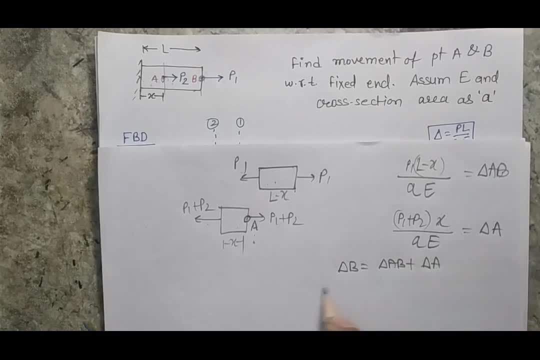 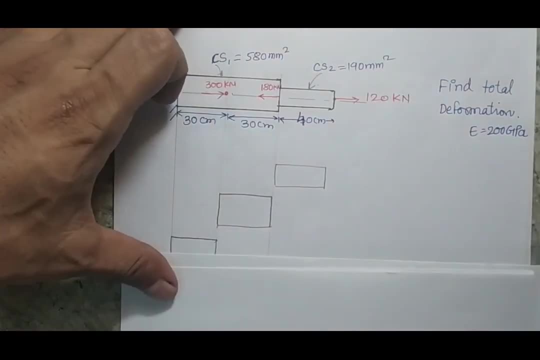 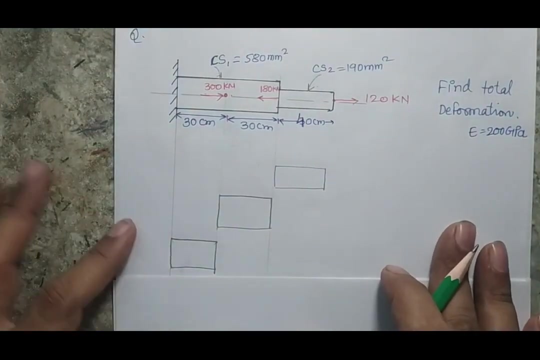 am interested to find the deflection of point b, that will be a b plus del a. so now let's solve a problem here. i am showing you a problem that i am having. instead of i am having the constant section bar, i am having a bar which is having variable cross section, and there are three forces acting here. 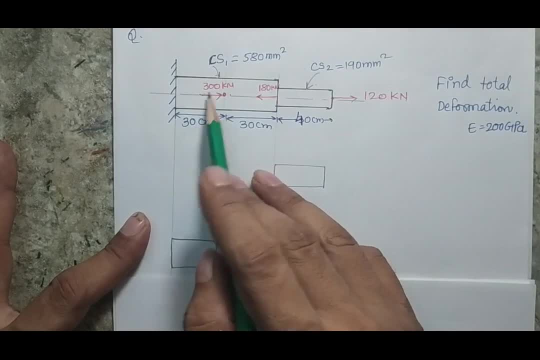 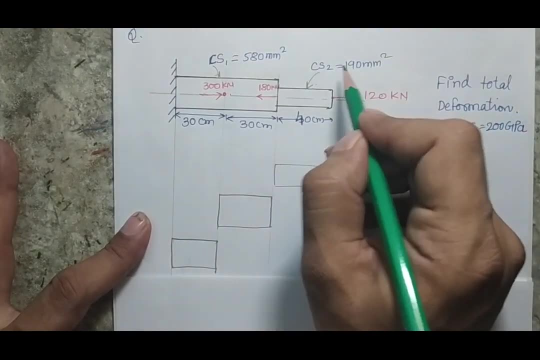 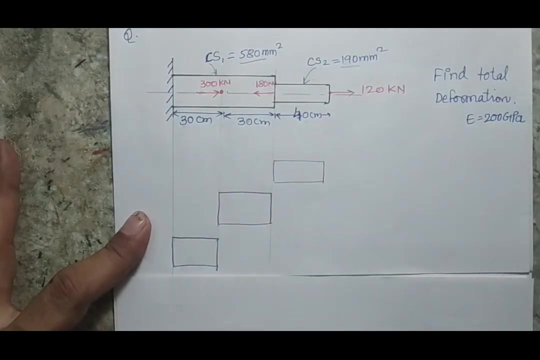 120 kilo newton, 180 kilo newton and 300 kilo newton. cross section: for this larger one is 540 and for this smaller one is 540 and for this smaller one is 540 and for this smaller one is 190 and this is 580, and the length are 30 centimeter, 30 centimeter and 40 centimeter. 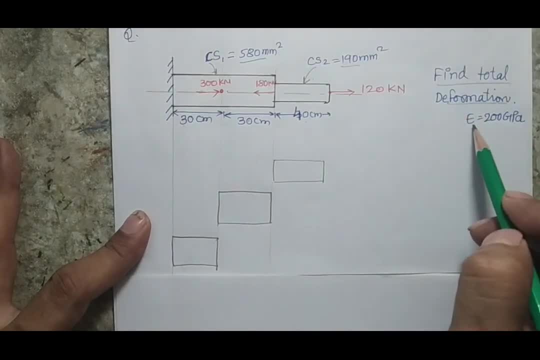 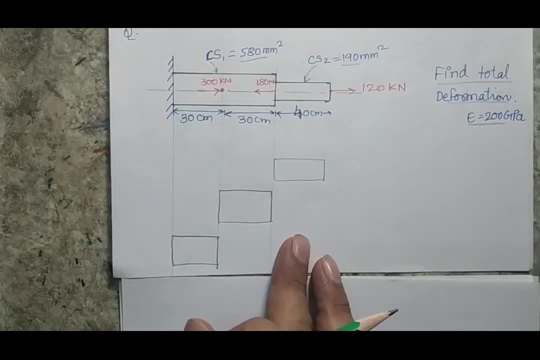 and i am interested to find the total deformation in the bar. elastic constant has been given as 200 giga pascal. so again what i need to do: first i have to find the forces in individual section so that i can find the change in length in the individual section. i will start again from here. 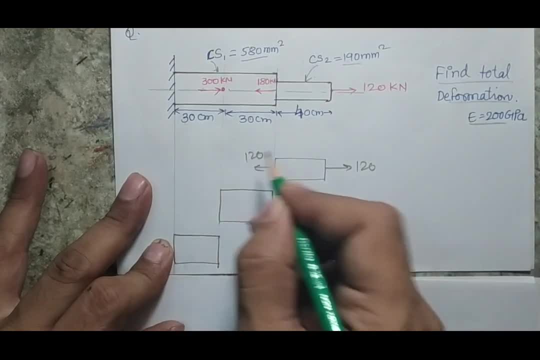 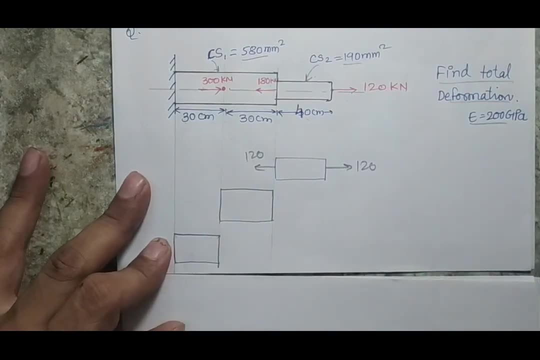 this would be 120. so this would be again 120. this is numerical values are exactly same, which i have already shown you in the previous video. so this is the change in length of a, b and this is the different in this particular section i have shown you in the previous problem. only the difference is. 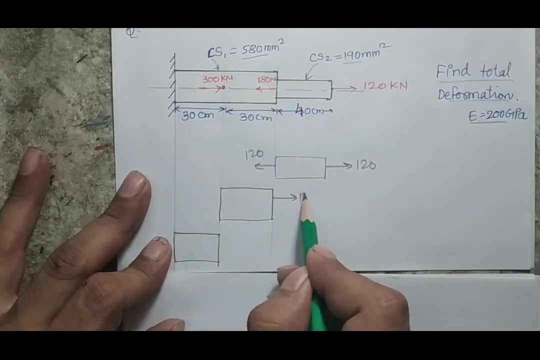 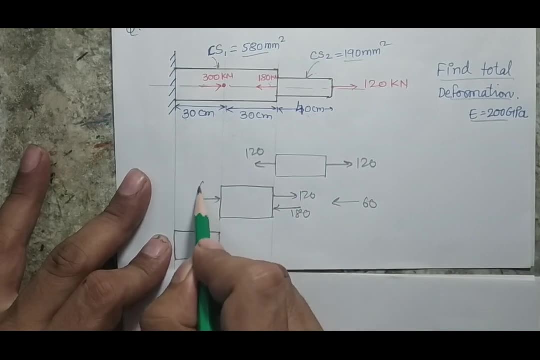 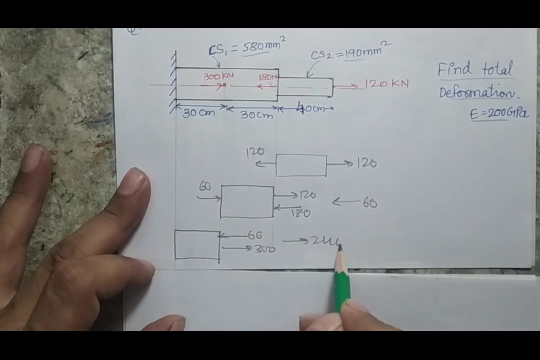 that i am having the change in cross section, the for the second section. i know that this would be 120 and this would be 180, so ultimately this would be a 60 force in this direction. so equivalent of this is 60 here, that this would be the 60 and this would be the 300. so i am getting a force of 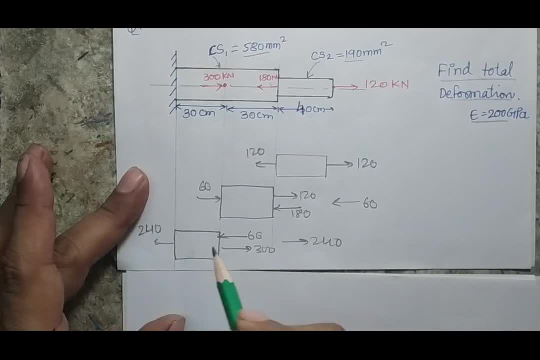 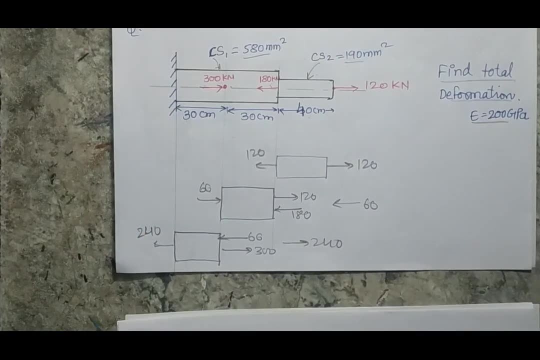 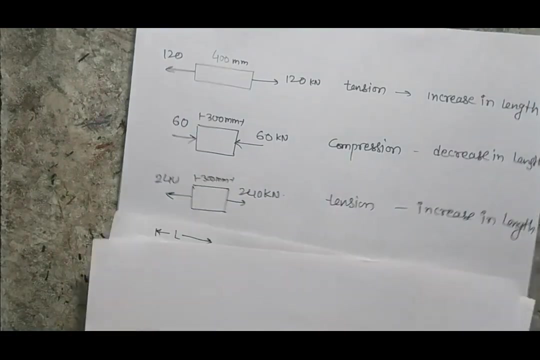 240 in this direction, so the 240 in this direction. so as now, i have find the, i have found the each cross section, and if I am interested to find the change in length of each cross section, what I can do, I can simply see here that this is my 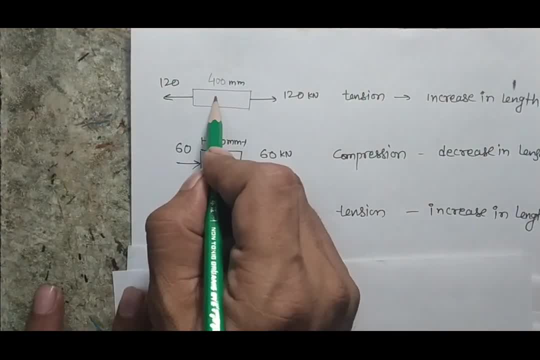 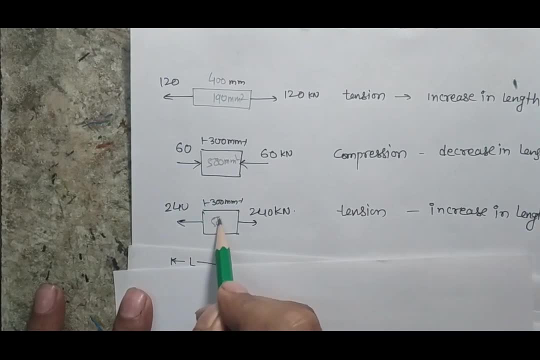 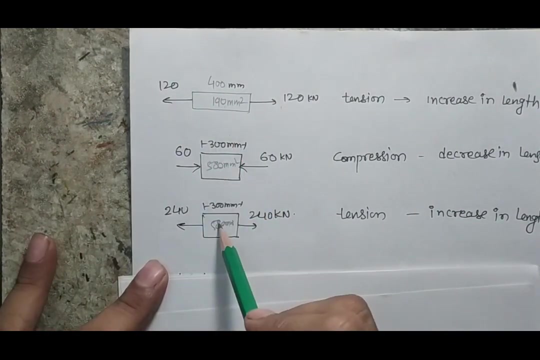 these are the three section where the cross section for first one is 190 mm square. for other section it is 580 mm square and 580 mm square. so I am going to put these forces for individual section. but I can see here that for the first section the forces of tensile nature, so that mean that there will be 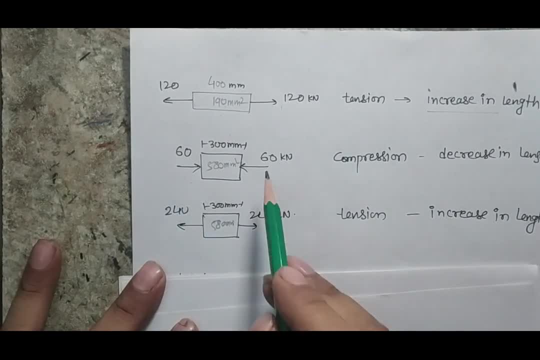 increase in the length. for the second section, the forces of of compressive nature, so definitely the length in change. change in length will be negative, or the decrease in the length, and for the third section, it is also again increase in the length. so if I am interested to find the total deformation, 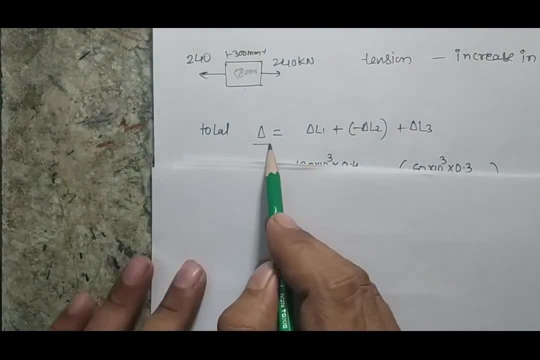 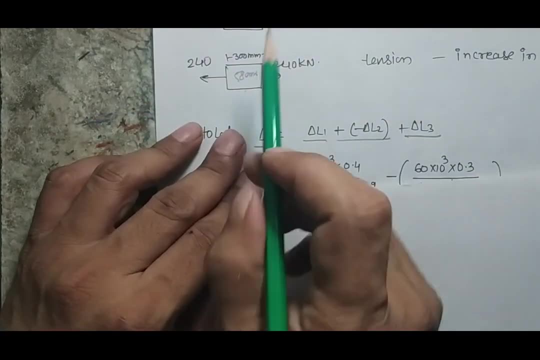 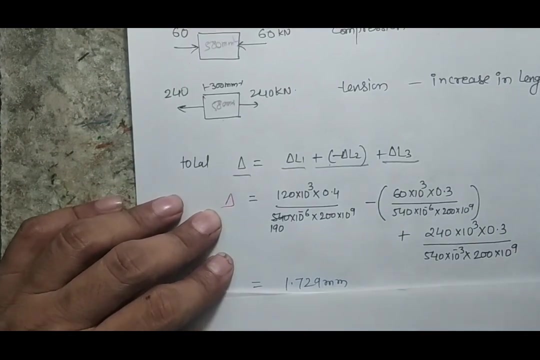 what would be my formula? my formula would become that the total deformation will be change in length in l1 plus l2 plus l3. now here either you can put- you can first calculate the change in length and then you can subtract, or you can simply put the negative sign for the forces value and you will get the same answer. 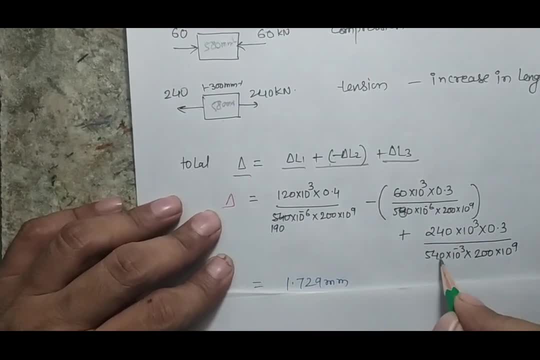 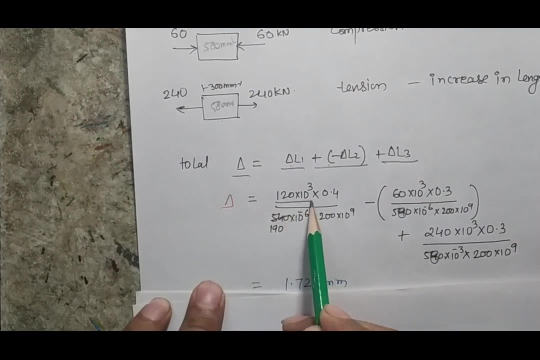 so these are. these are the numerical value. this is 580 actually. so now, this is for the first change in length: 120 kilo Newton, so 120 into 10 to the power 3. this is the length of the bar. this is the cross section of the body and this: 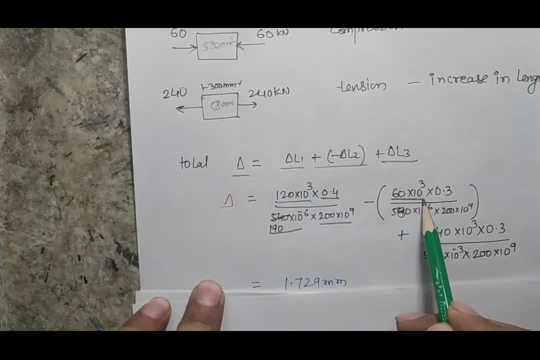 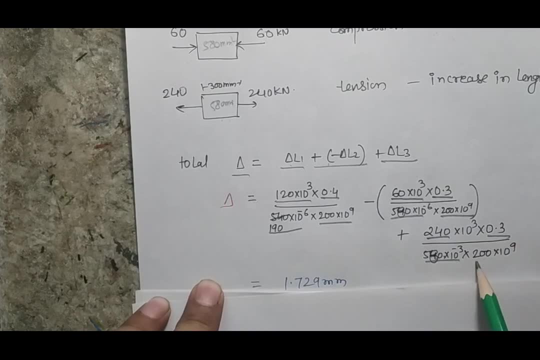 is the elastic constant. similarly for the cross section of the body, this is the nghw and historic determine and initially for the second force is 60 kilo Newton. this is your length cross section and the elastic constant. and similarly for third force: length, cross section and the elastic constant. when I 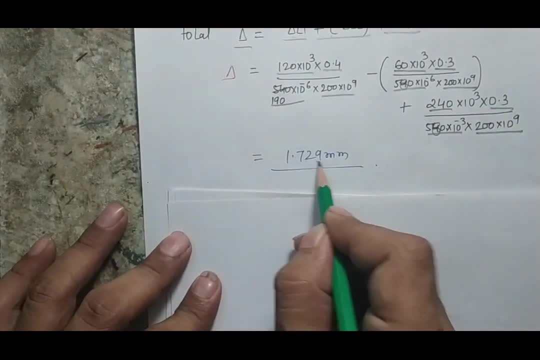 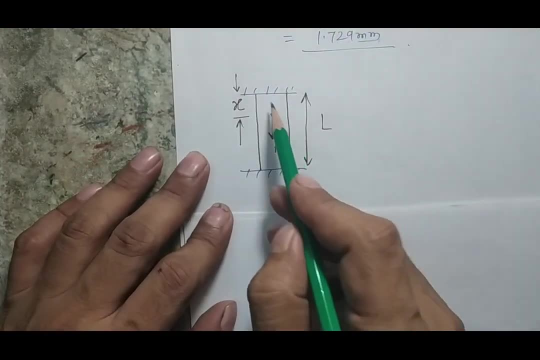 will solve the problem. I am getting an answer that the total change in length in 1.7 to 9 mm. now in the last I am showing you, showing you a problem here: I am having a bar which is fixed at both the ends and I am applying a force P at 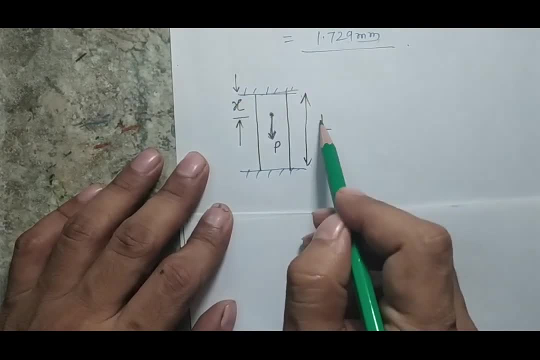 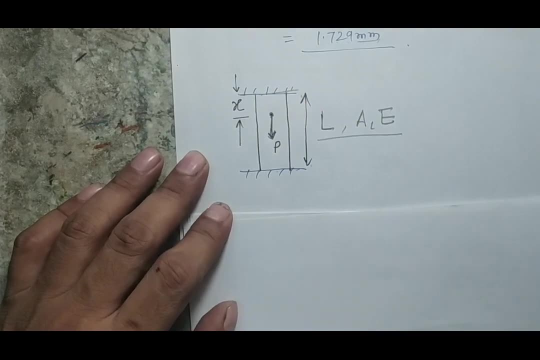 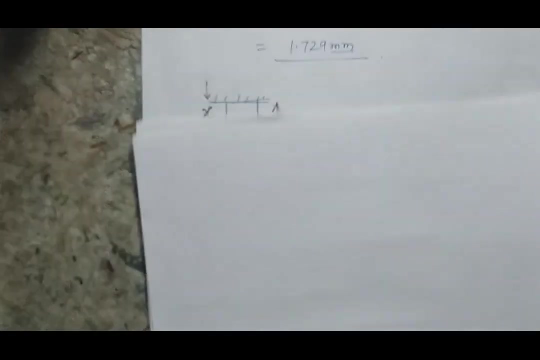 x from the top fixed end. the total length of the bar is l. suppose the cross section area is a and the elastic constant is e. so do you think that by applying the similar philosophy which we have already done, solved in this problem, we will be able to get the total deformation in the 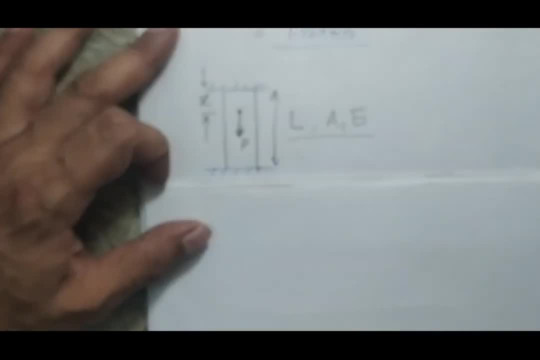 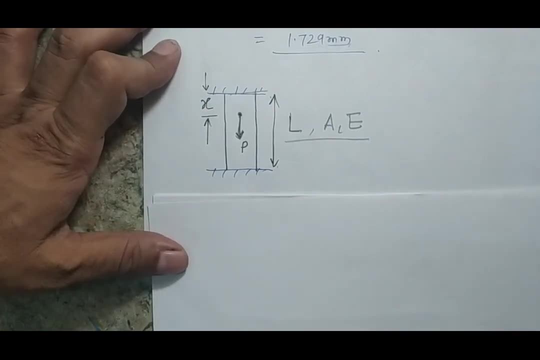 body or we need something more. so when we will see this problem in detail, we will observe that this is not a simple case, whatever so far we have solved. that is called the problem, which is statically determined by using the free body diagram. we can find the forces in the system, but 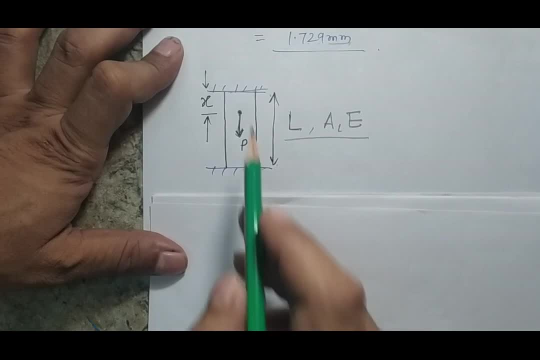 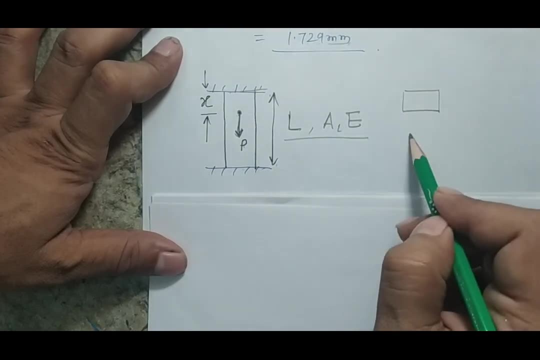 in this case, if you will try to find the forces in the system, what you will see? that suppose this is the force p. so first question: it should be in your mind that the forces in the top part and the forces in the bottom part would be p, p or something else. so the force p is applying here at that means that 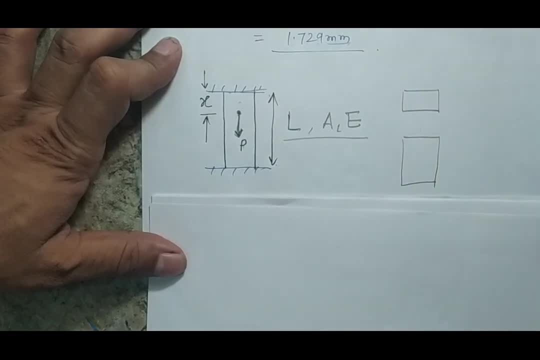 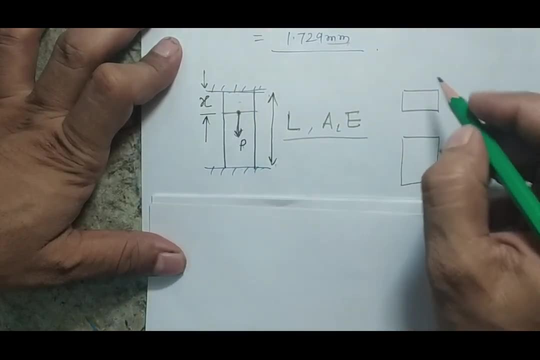 the, not the top and the bottom portion are having the same force p p. some of the portion would be there by the top portion. suppose that this portion definitely would be in the tension. so i am assuming one reaction r1 here as i am resuming reaction r1 here. so definitely this. 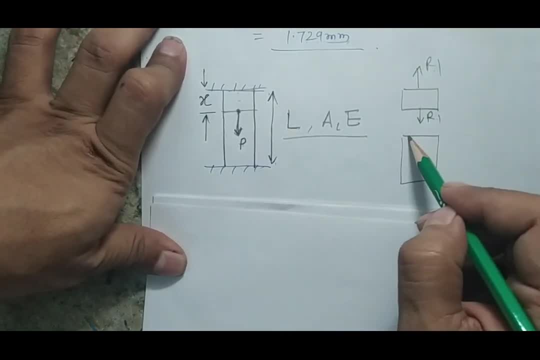 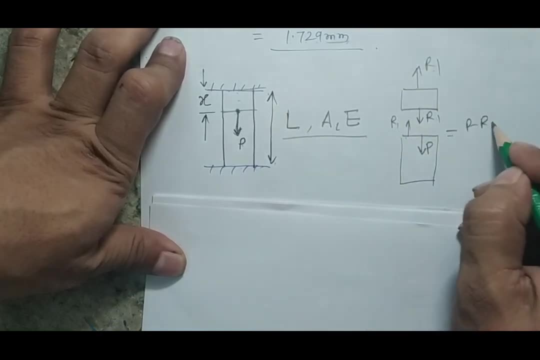 would be my r1, as i know that this is r1. so there would be one force r1. instead of that, another force, p, is also acting here. so. so net force here will be what p minus r1. that would be in downward direction. so another force will be what p minus r1. so here, if i am interested to find the force p, 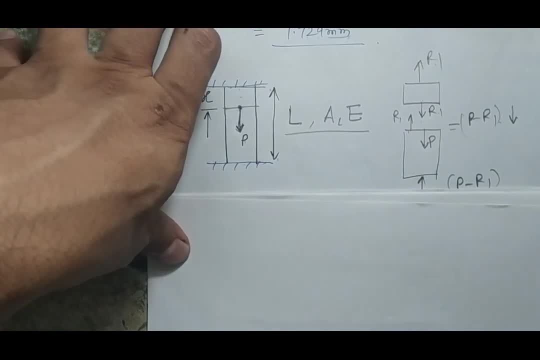 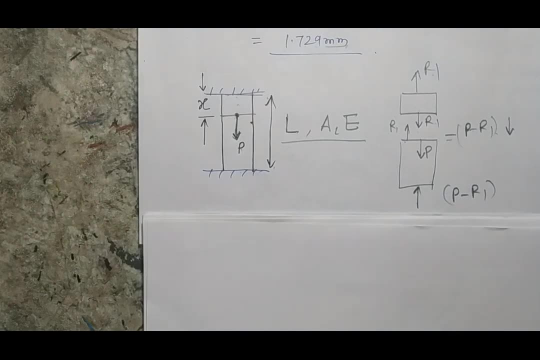 and the change in length of the body. i need something more and such kind of problem we are going to see when we are going to see the section where the statically indeterminate problem which we will see in our next lecture. thank you.